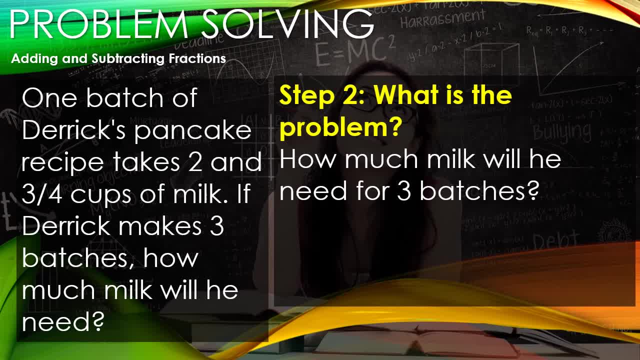 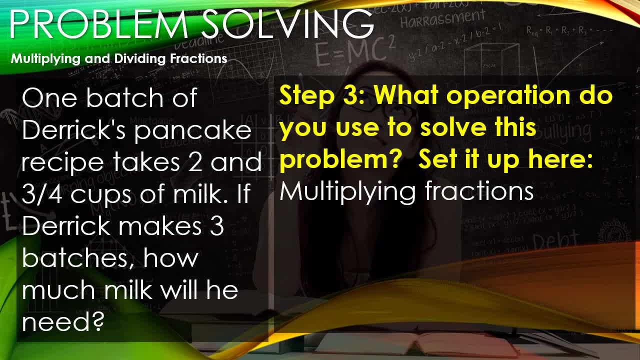 how much milk he needs for three batches. So, in order to do this, our operation we're going to use is we're going to multiply these fractions together And then the second little part here are fractions. So we said it's multiplying, So we have two and three, fourths times three. 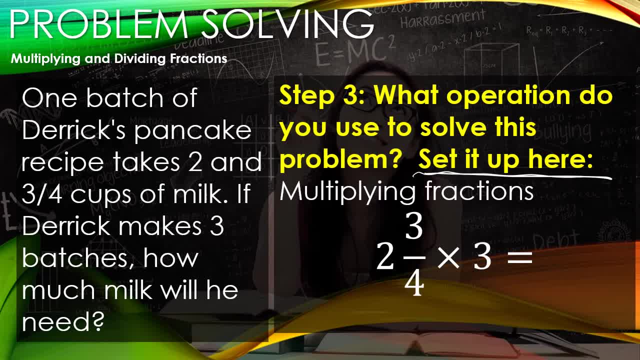 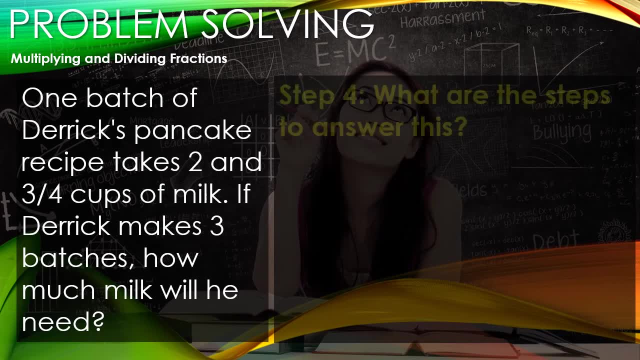 And you notice we are here at step number three is we are slowing you down so that you can read the problem, figure out what operation it is and set it up correctly before you even try to start solving it. So now we're at step number four, which we're just going to write out. the 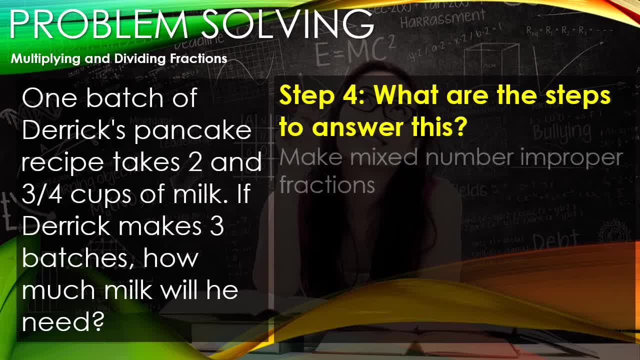 steps that this is going to take to solve this problem. So we're going to start by writing out the problem. So, when we're multiplying fractions, our first step is we're going to make the mixed numbers into improper fractions. We're going to make the whole number into an improper fraction. 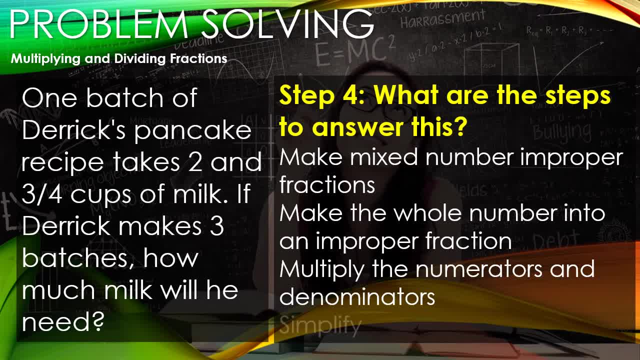 We multiply the numerators, we multiply the denominators and then we simplify. So we have some steps here, But we're at. step. number four is we're figuring out what our steps are. So we're so close to figuring this out here, And so we have what we drew. 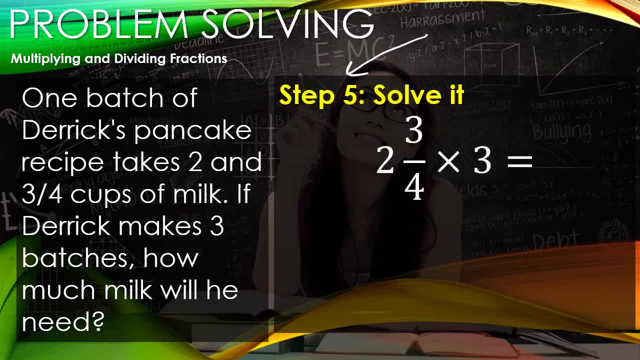 we wrote out two and three, fourths times three. Our first step is: let's go ahead and make these numbers into improper fractions. So we can do four times two is eight plus three is eleven, So I have eleven fourths times, and then make our whole number three into an improper fraction is just. 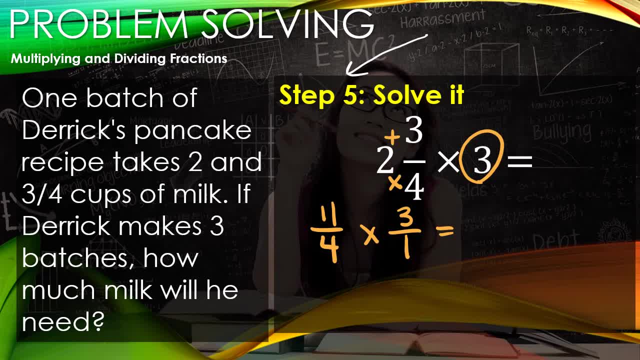 three over one. Our next step is: we're going to multiply our numerators together. So eleven times three is thirty-three, And four times one is four. So we have this improper fraction We're doing so good. We just got a couple more things we got to take care of. Let's go ahead and change our improper fraction. 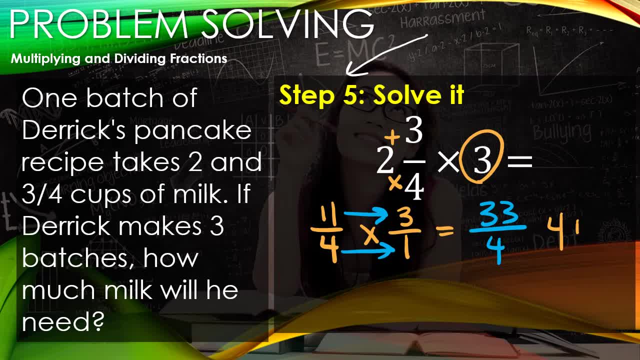 into a mixed number. The way we do this is we do some fancy long division here. Four goes into thirty-three, eight times, And we have a remainder of one, And so the way this works we have our whole number is eight. So that's our whole number. We keep our denominator the same, So our denominator is four, And then the. 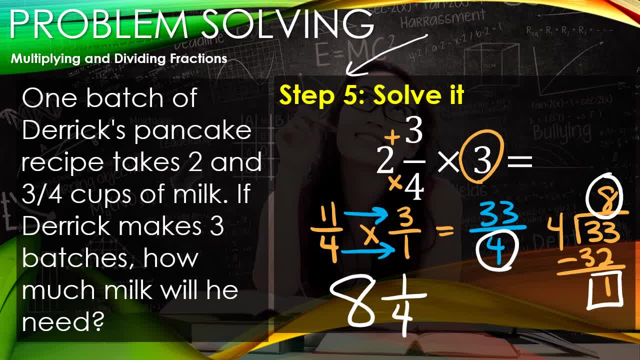 last little bit is this remainder of one. That's our numerator, And so we can say that overall, how many cups are required for this project? We can say there's eight and one fourth cups, And the way we can kind of double check to make sure we're so close to being on the right track is if we 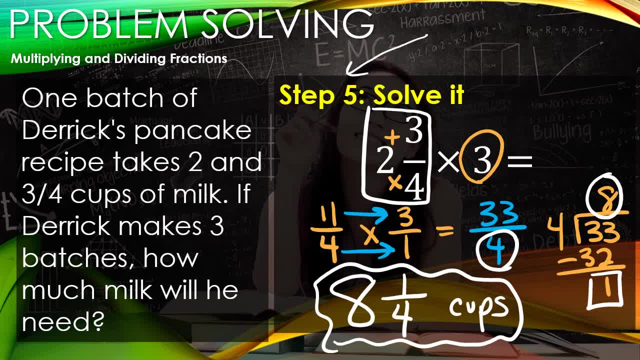 can estimate two and three fourths. We can estimate that to be three. if we round that up, If we multiply three times three, it gives us nine, And so we kind of can know, based on our estimate, that our number eight and one fourths is a very reasonable answer. It is the correct answer for this problem. 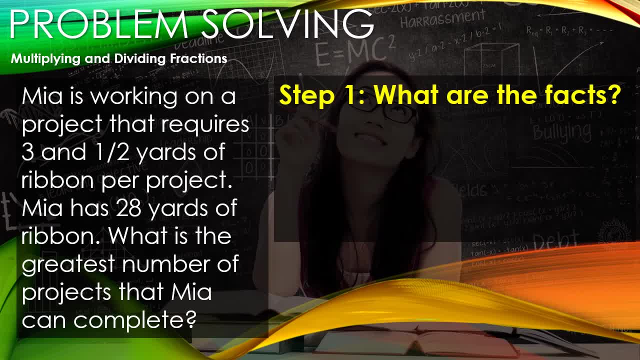 So let's try a second problem here. So our friend Mia. she's working on a project that requires three and yards of ribbon per project. Mia has 28 yards of ribbon to start with. what's the greatest number of projects that Mia can complete? so, first of all, Mia is making 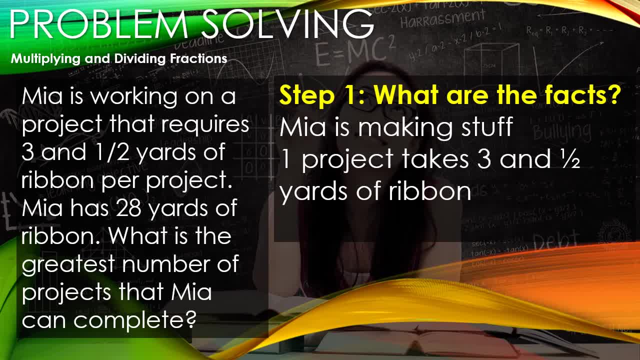 stuff out of ribbon. so our second fact here is that one project takes three and a half yards of ribbon. so whatever she's making- whether it's a bow in her hair or she's making a pretty border around a project- whatever she's making out of ribbon, one project takes three and a half yards of ribbon and she has 28. 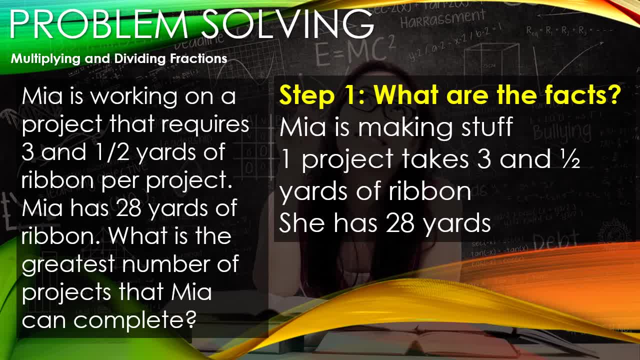 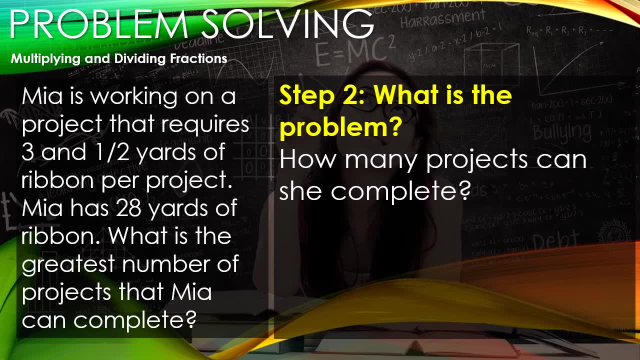 total yards to start with. so she went to Michael's or joy and fabrics or Hobby Lobby, wherever she went- and she purchased 28 yards of ribbon and she's thinking, hmm, the question was how many projects can I complete by making a project out of ribbon with my 28 yards of ribbon? so remember, each project is three and a half yards. so 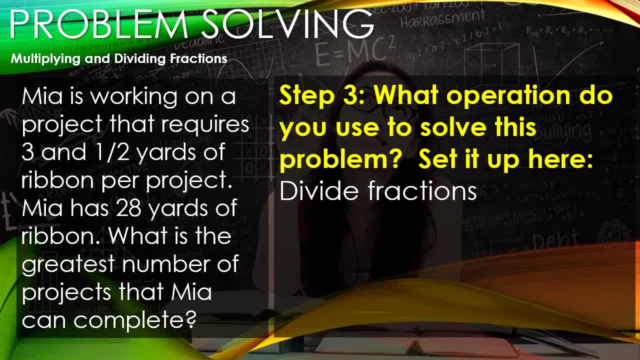 what we can do. the operation we're gonna do this is we're gonna divide these two numbers. the way we're gonna set this up is we have the total number of yards- she's starting with this 28- and she's gonna divide that or cut that knit for. 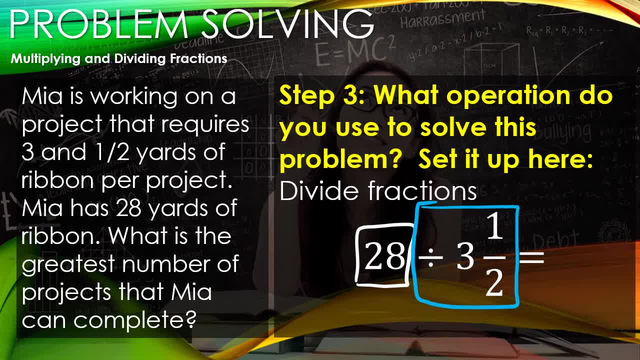 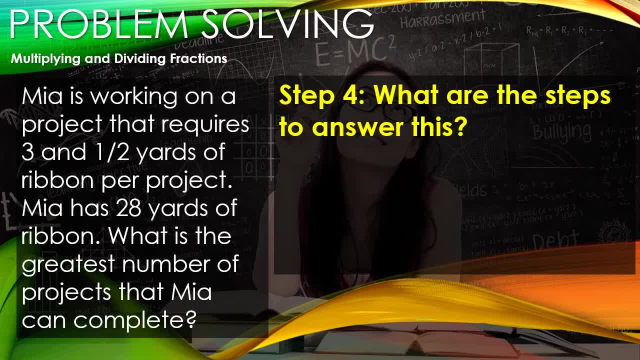 each project being three and a half yards. and so for step four, just remember, we are so close, we have some great information going on and we are so close to completing this word problem, so we know that our steps are. we're making all of our mixed numbers into improper fractions and for 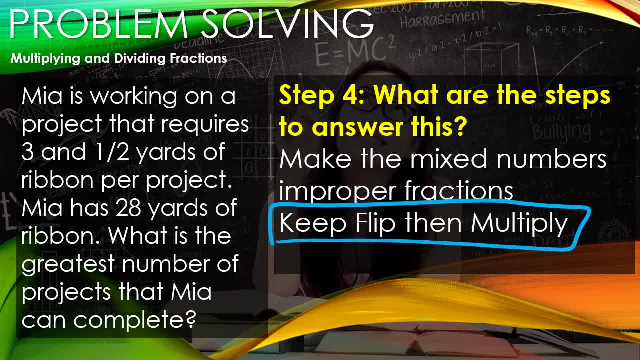 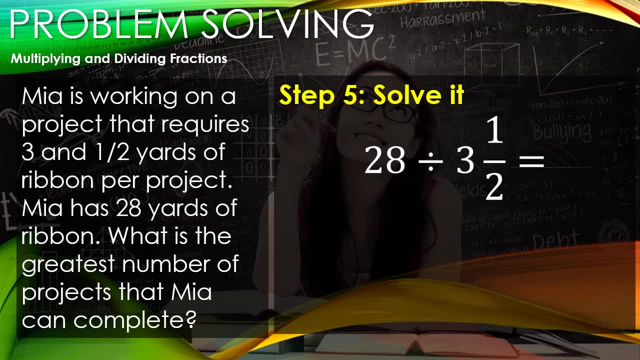 division. we're gonna keep the first fraction, we're gonna flip the second fraction and then we multiply them together. and I wrote over top of the words simplify. so now step five, step five is we're going to divide these two. all we have left to do now is to solve this. so our very first step is: we're. 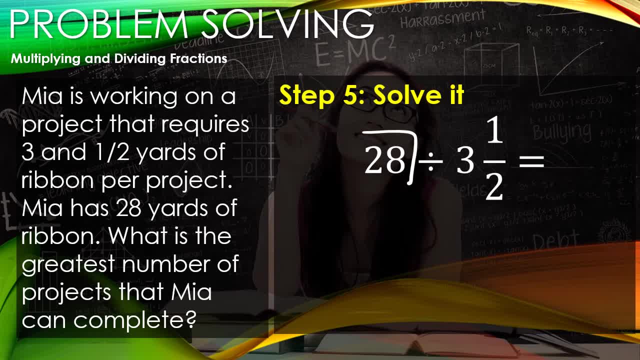 going to make everything into improper fractions. so 28 as an improper fraction is 28 over 1, and we're going to divide that by 2 times 3 is 6 plus 1 is 7. so 28 over 1, divided by 7 over 2. and now what we're going to do is we're going to 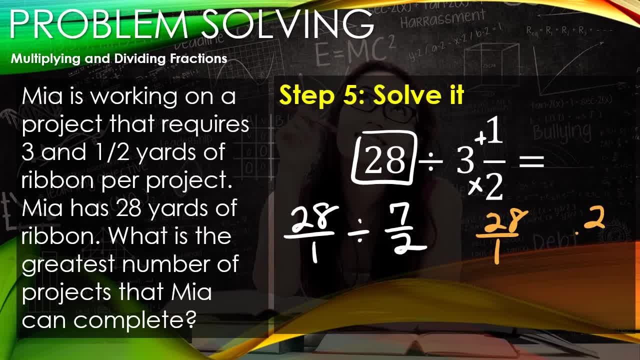 keep our first fraction, we're going to flip the second fraction and you guess that now we're going to multiply. so when we do this, so 28 times 2 gives us 56 over 7. and to figure out what this improper fraction is as a mixed number, we can do: 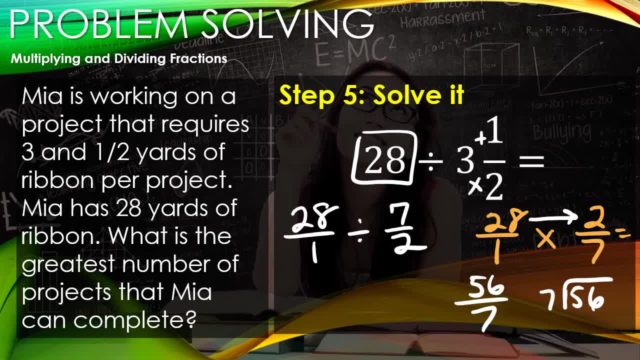 7 goes into 56 and we have 8. 8 times 7 is 56, with zero remainder. and so, to figure out the number of projects that she can complete, she can complete eight total projects and you might say you know that's a lot of steps. 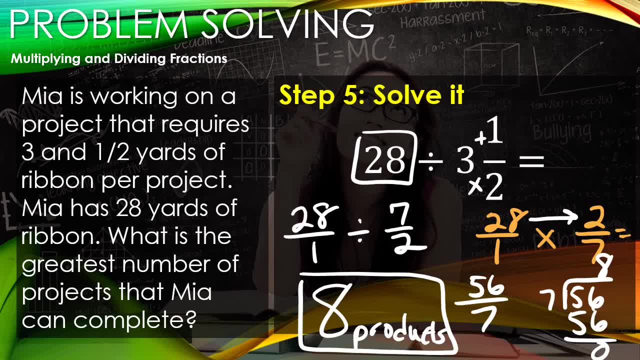 how did you get there? how did you do that? and so what we can do is we can take a look at. what we have here is, if we rounded 20, uh, rounded three and a half, to, let's say, we round it down to three. so if i did 28 divided by three, that gives us a little over. that gives us about a little over.